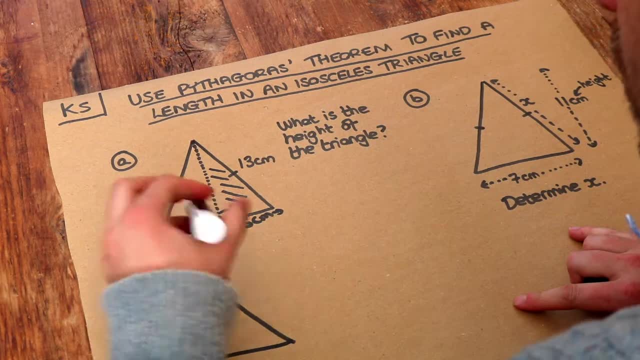 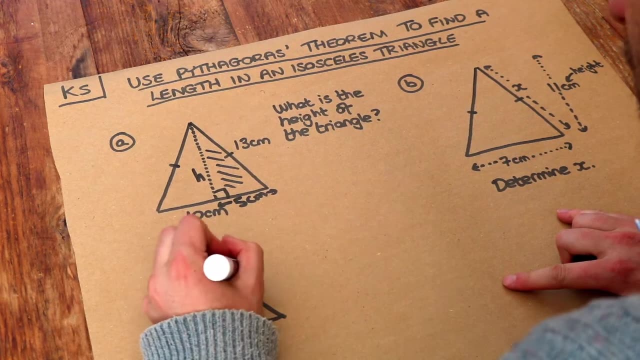 So let's draw that triangle separately. We've got the height here. let's call it h. We've got that 5 centimeters at the bottom and we've got this 13 centimeters here. So let's use Pythagoras Theorem. 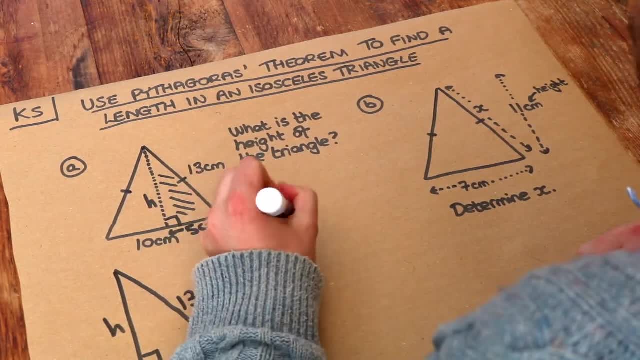 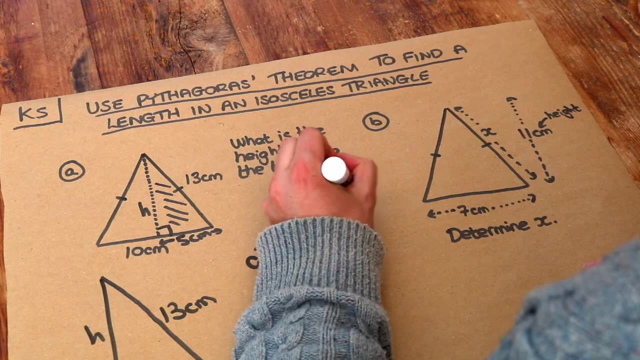 We saw in a previous video that Pythagoras Theorem is just a squared plus b squared equals c squared, where c is the hypotenuse the longest length of the triangle. It doesn't matter which way a and b go around, So let's just call this shorter length, a. 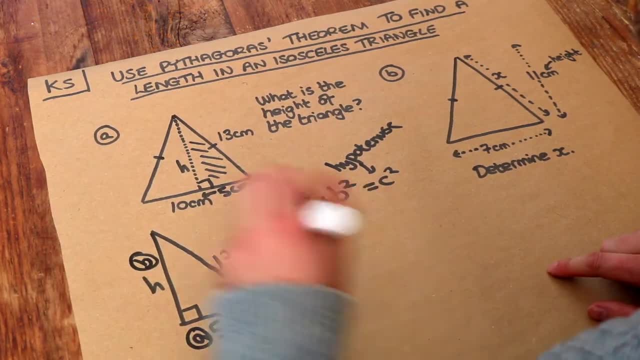 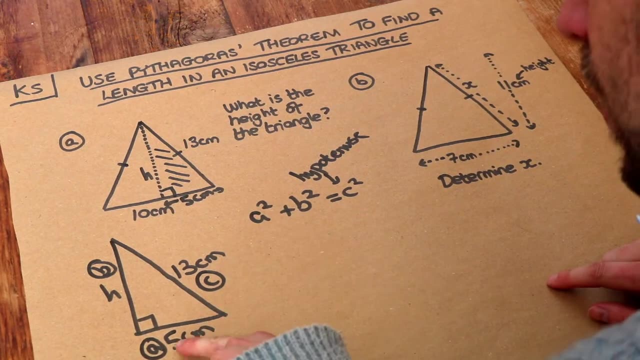 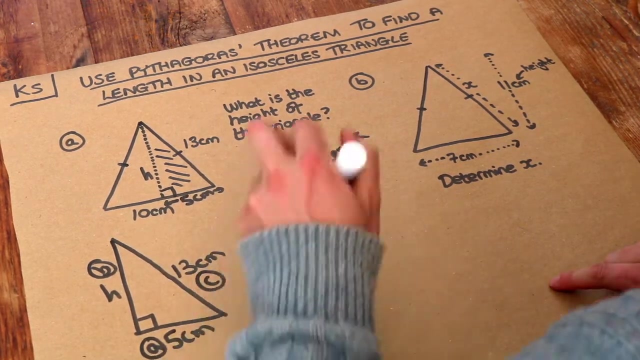 this shorter length, b, and then the longest length has got to be the c. As I said before, it doesn't matter which way a and b go around, but let's substitute these into the formula. We've got a squared, 5 squared, plus b squared, which is h squared, is equal to 13 squared. 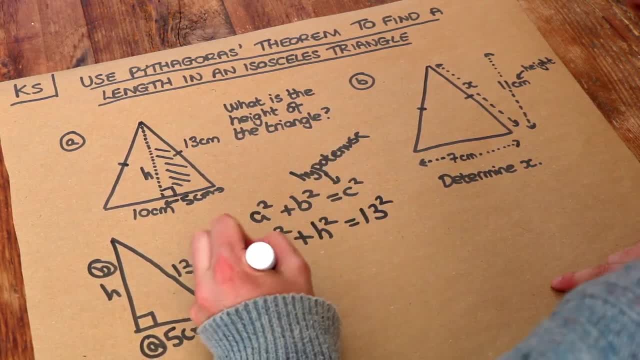 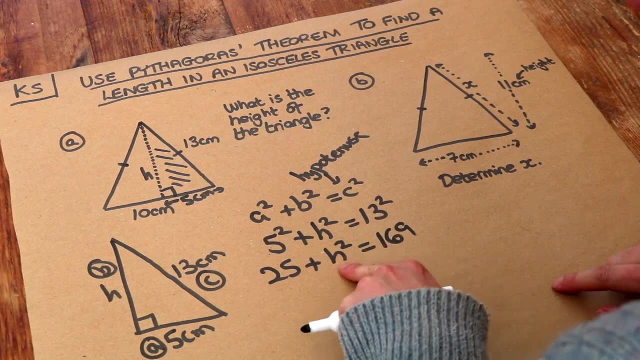 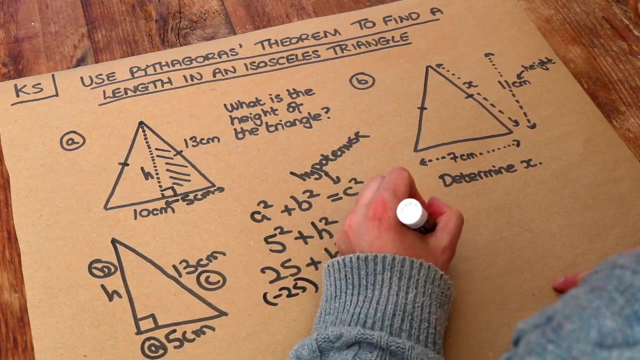 Then let's just work out what 5 squared and 13 squared are. that's 25 plus h. squared x equals 169.. Now h is being squared, then we're adding 25 to it to get one, six, nine. so we should subtract 25 from both sides to get rid of the plus 25.. 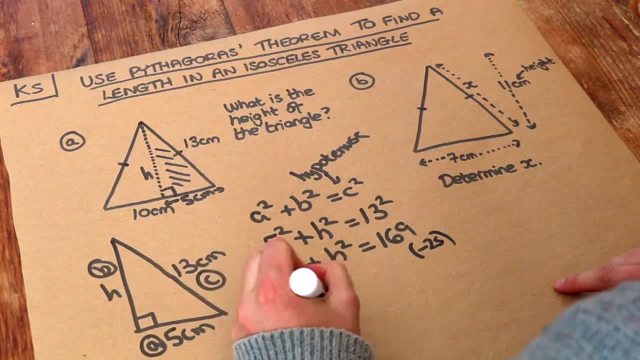 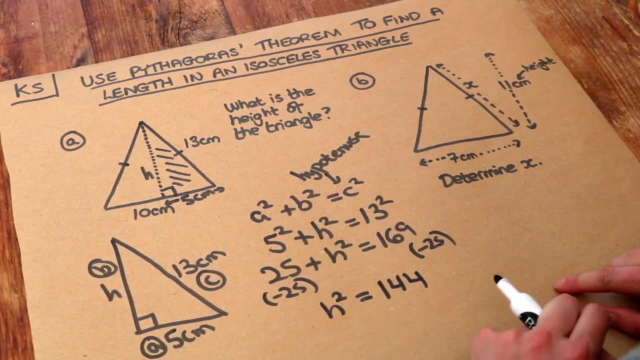 The minus 25 gets rid of the plus 25, rid of that plus 25, leaving just h squared. and then 169 minus 25 is 144.. Now h is being squared to get 144. we want to undo the squared, so we square root each. 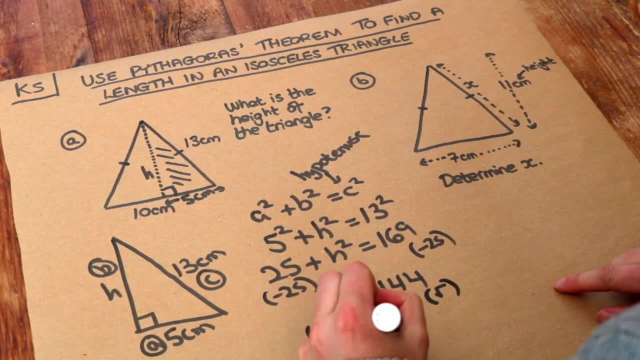 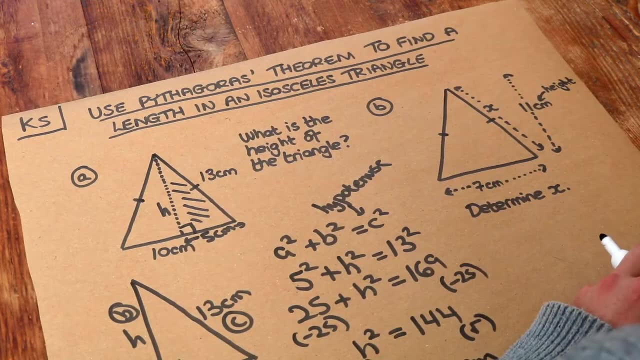 side of the equation and that gives us h is equal to 12 and it's going to be in centimeters, isn't it? because the other units in centimeters? And that's the final answer. we've worked out the height of that isosceles triangle. What about? 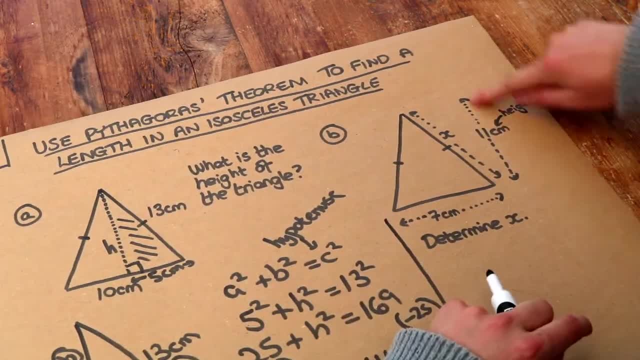 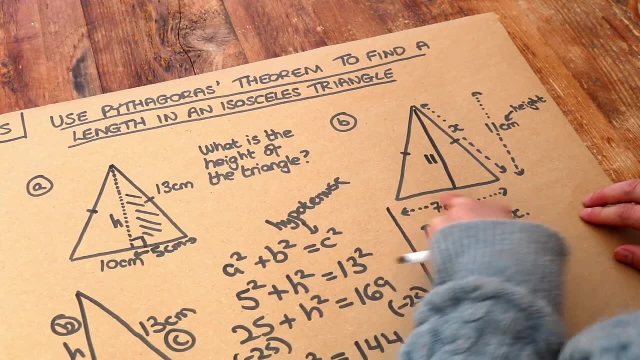 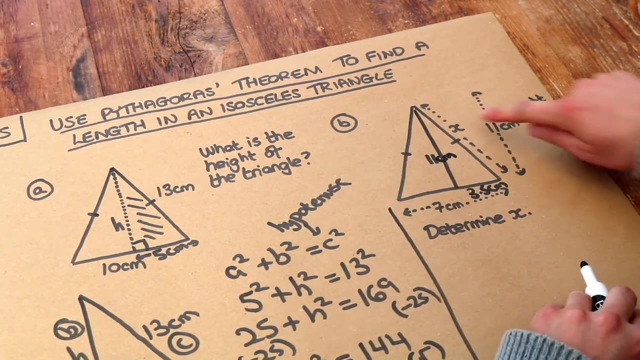 this second one. Now we're told the height is 11. so I can put this 11 in and we've got the bottom length is 7. if we split that in half again that's going to be 3.5 centimeters here and we want to find the hypotenuse X. so if I draw that, 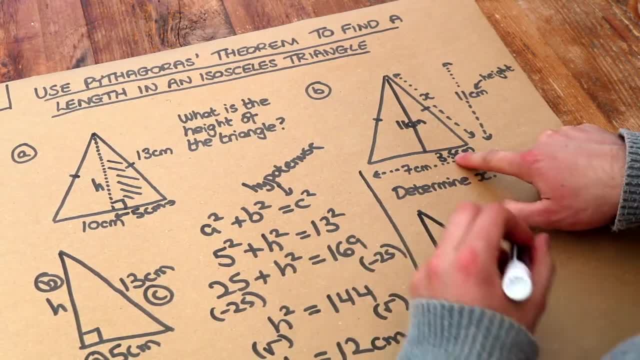 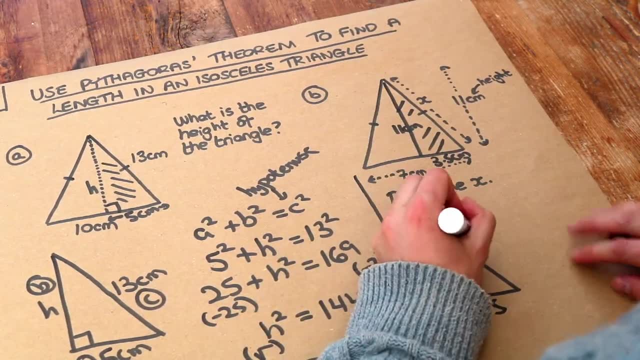 triangle out separately. again, we've got the 3.5 at the bottom, we've got the 11 going up the height and we want to find that slant height. so, using Pythagoras theorem, again we do one: the shorter side squared, so the 3.5.